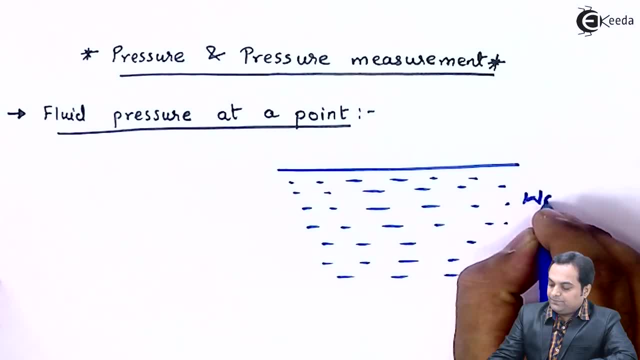 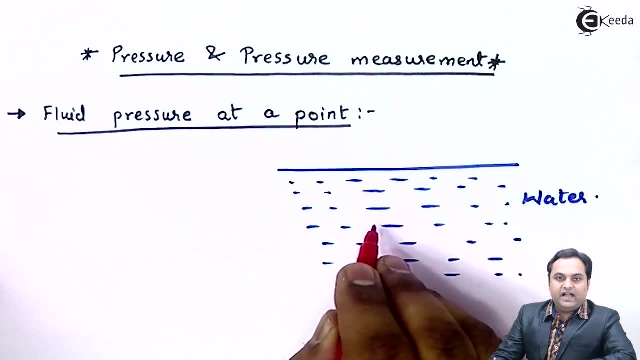 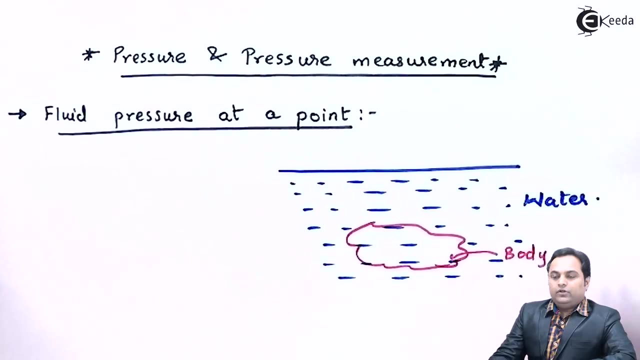 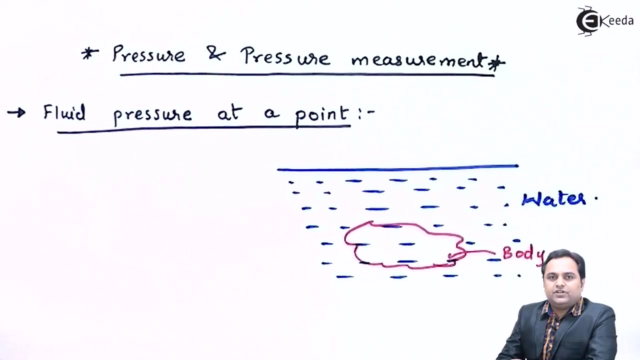 I am assuming that this fluid is water Inside this water, if we have a body of any given shape, So there would be a pressure acting on this body. Now how this pressure would be acting, Suppose if I take a very small area of this body. 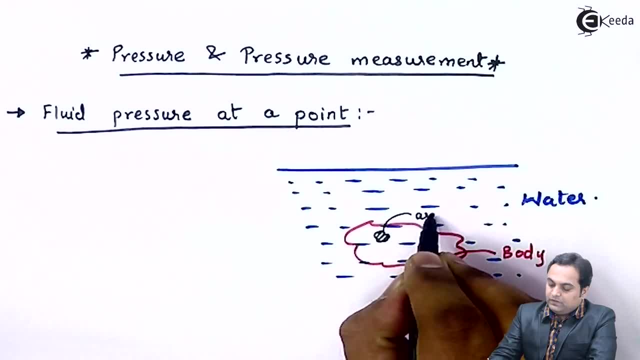 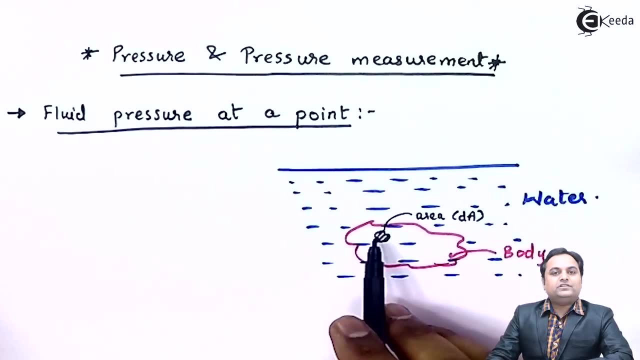 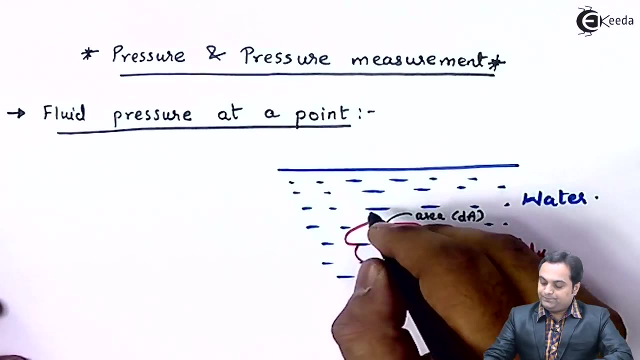 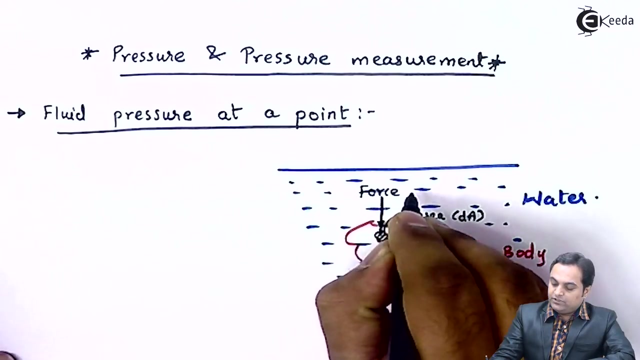 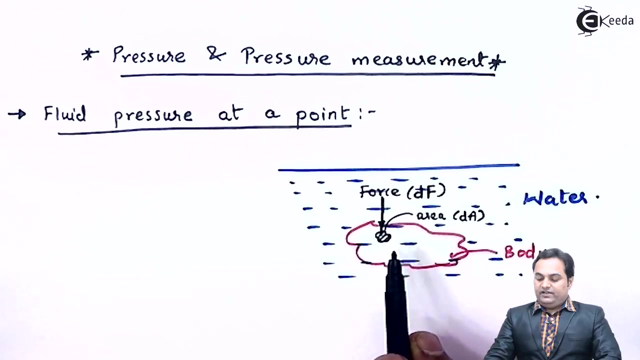 I will call this area as dA. that is a small amount of area. Now, over this small amount of area, a small force would be acting. That force I am denoting here, It is denoted by force dF. So now, when a force dF acts on an area dA, 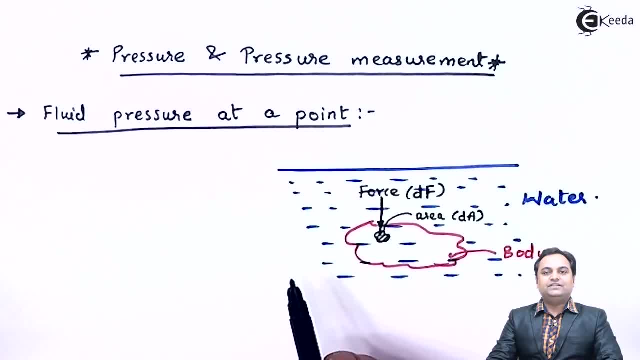 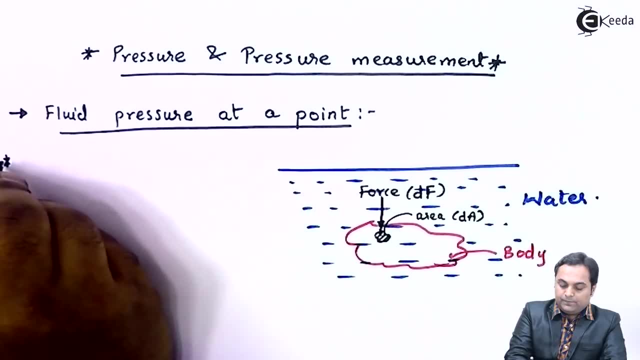 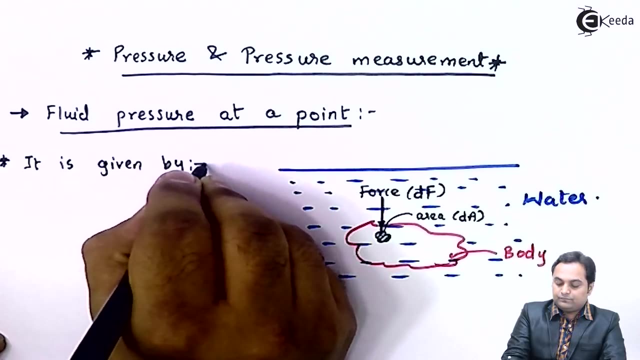 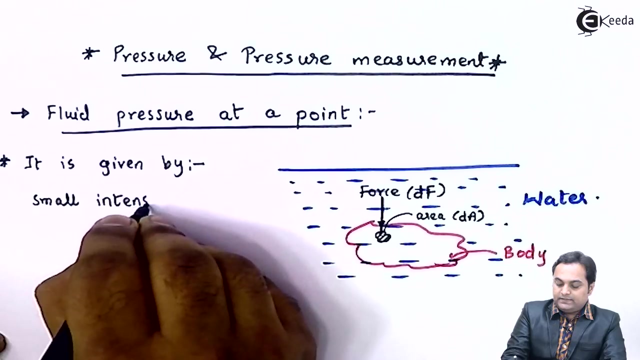 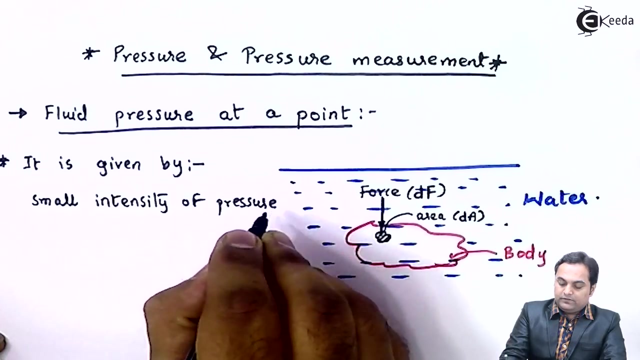 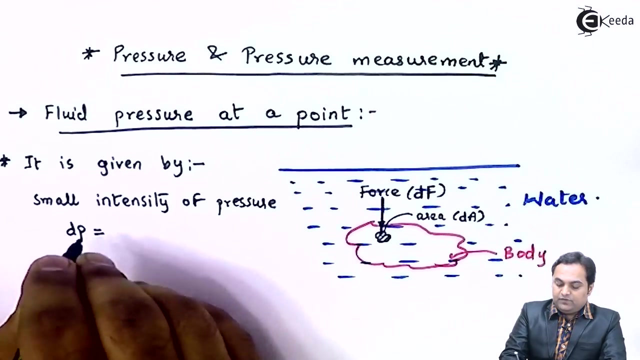 That would be called as intensity of pressure. So finally, the fluid pressure. at a point It can be said that it is given by small intensity of pressure. small intensity of pressure That will be denoted by dP, small intensity is equal to- it will be given by small amount of force, which is dF. 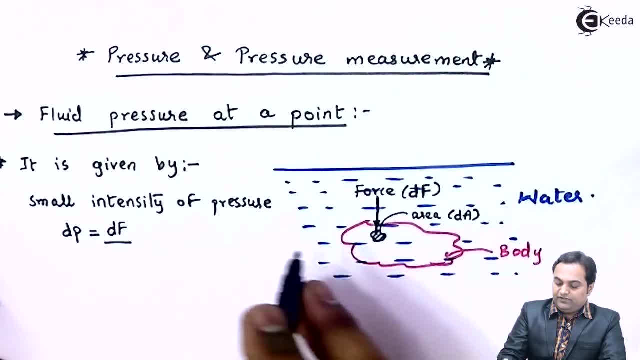 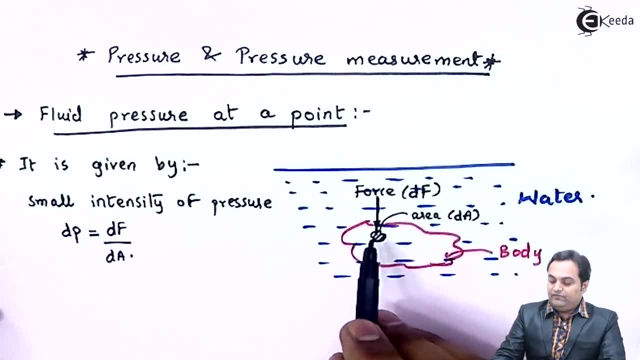 divided by small amount of area, that is dA. So this is the small intensity of pressure which is acting on small area. dA Now, if I consider the total area of the body, which is capital, A, So the force which would be acting on this body. 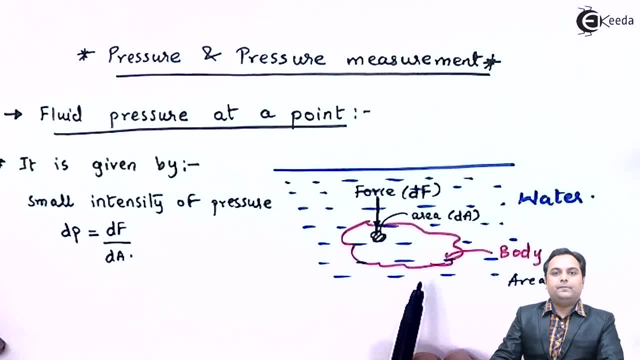 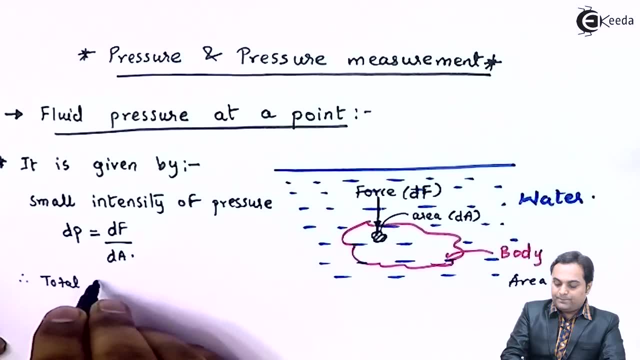 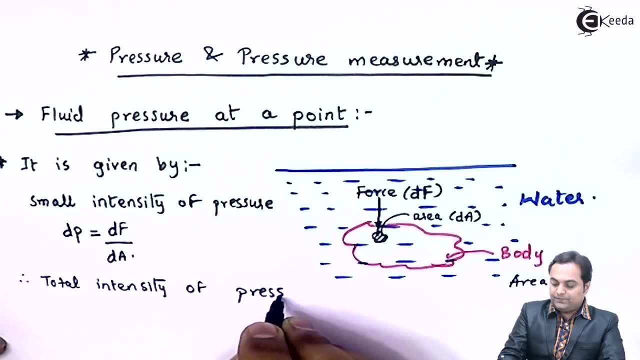 having area capital A would be denoted by capital F. So, finally, I will say that, therefore, total intensity of pressure, total intensity of pressure that will be given by, instead of dP, that is, small pressure, here I would be having the total pressure denoted by letter P.